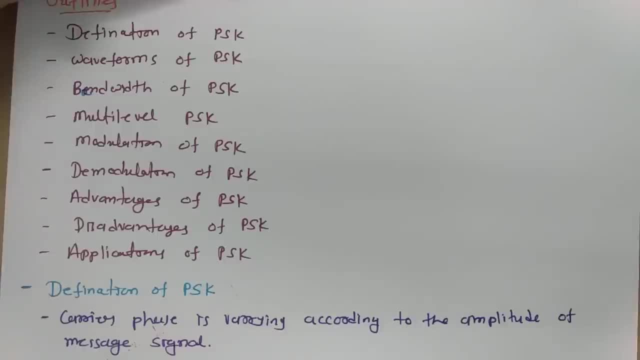 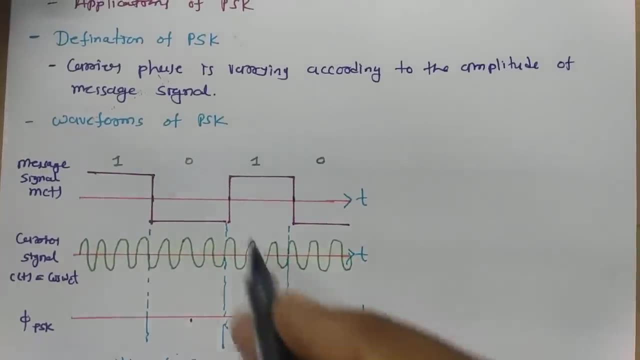 So this is what the basic definition that is there with PSK. Let us try to understand how phase is getting changed with respect to amplitude of message signal. So here we have message signal MT. This is my carrier. signal CT, that is cos, omega CT, And here I'll plot PSK waveforms. 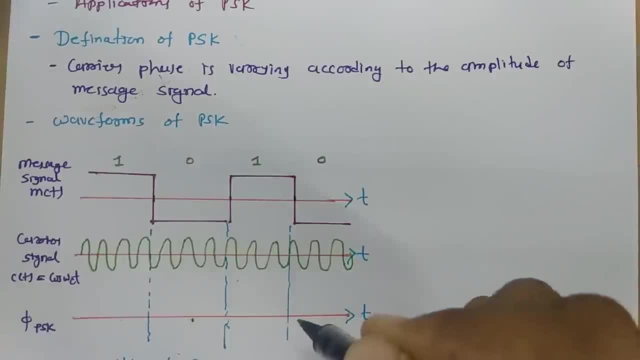 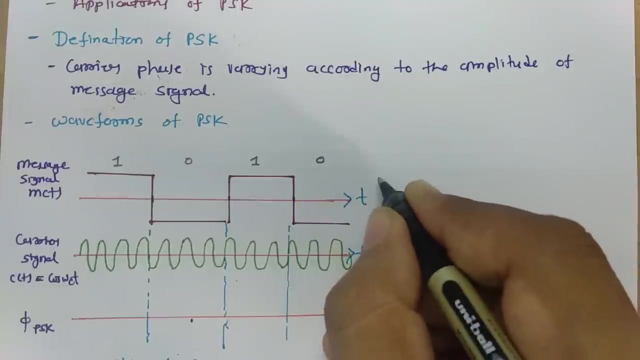 So see, before I explain how this waveform is there, we need to understand Here we have digital signal, So that digital signal that will be there in terms of 1s and 0s, And here I have drawn polar waveform of digital signal. So this is what polar waveforms of not return to 0. 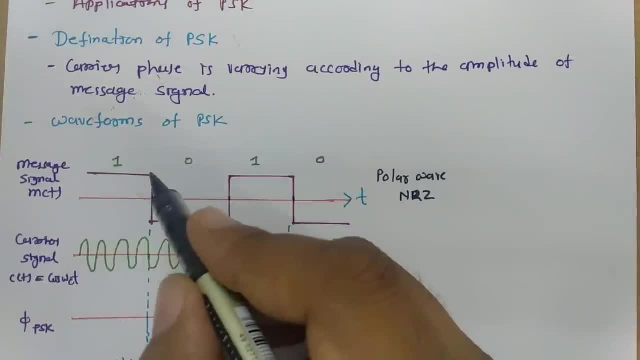 So in that for 1, there is plus amplitude And for 0, there is minus amplitude. So in that for 1, there is plus amplitude And for 0, there is minus amplitude. So in that for 1, there is plus amplitude And for 0, there is minus amplitude. 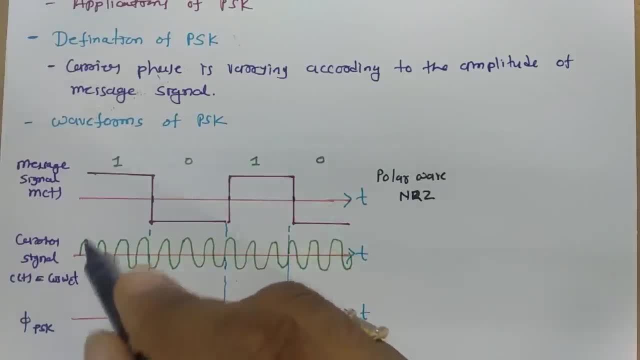 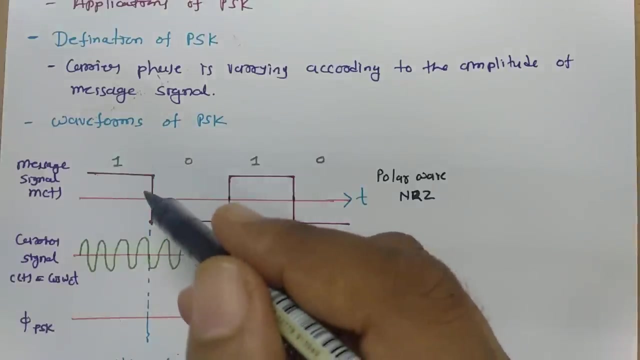 So that one can see- And this is my carrier signal, that is high frequency signal, And that high frequency signal that we are using it to translate this message signal into high frequency signal. Now see what will happen here in PSK phase of carrier signal will change with respect to message signal. 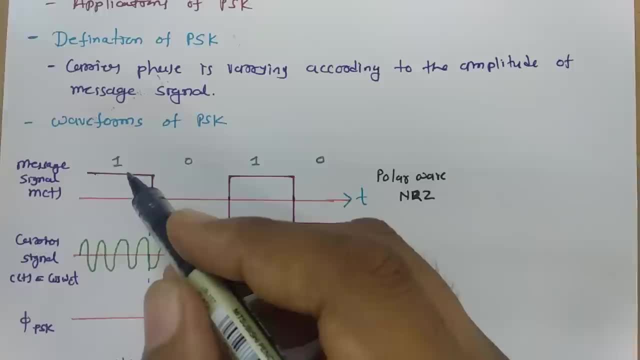 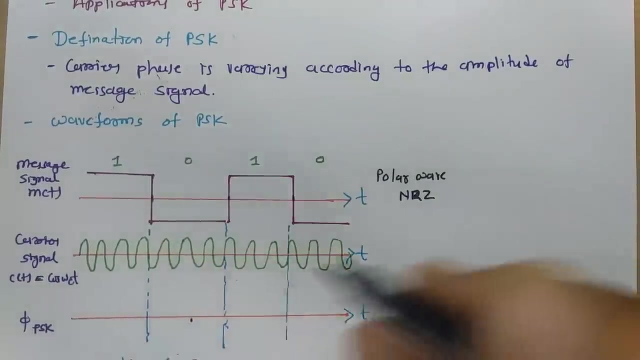 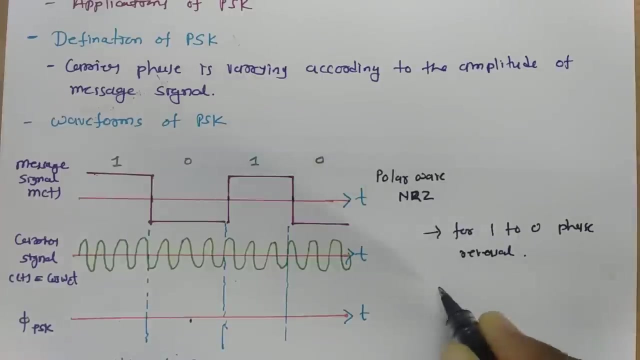 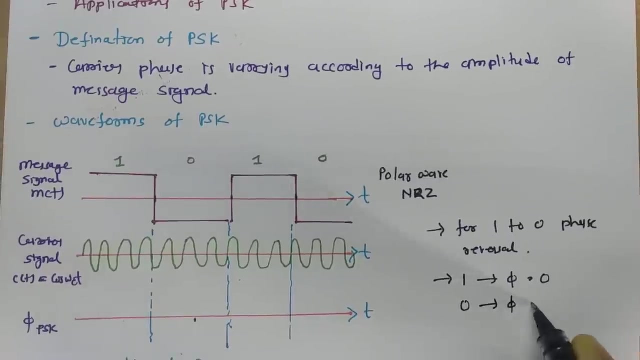 So whenever there is 1 at 0., At that time there is zero phase and for zero there will be a phase reversal which will happen. Like see, we can say for one to zero there will be phase reversal. or one can say for one: if phase change that is zero, then for zero there will be phase, that will be getting. 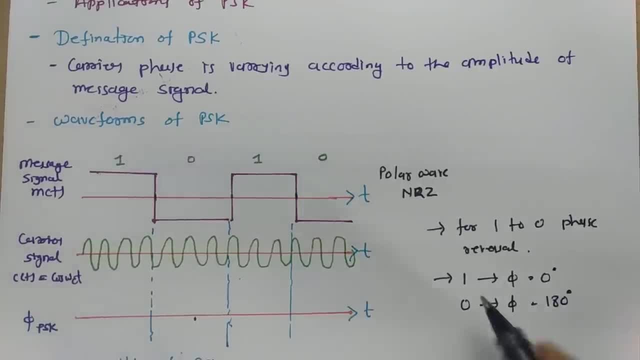 changed to 180 degree. So ultimately here, as if I say one, that is what I am translating: transmitting, in that case I will be sending carrier signal only, but when there will be zero that we are sending, at that time there will be phase reversal. So see, when there is one at that time, same carrier. 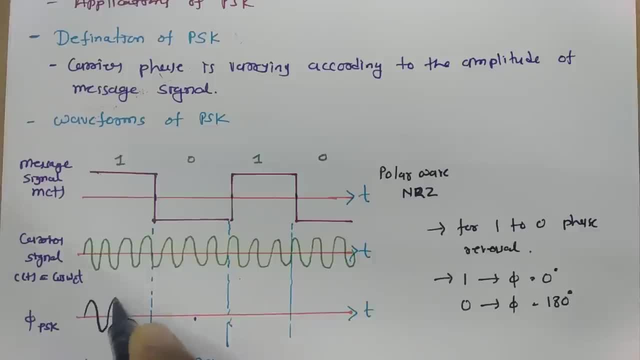 signal that we will be sending. Let us say this is what for one now, then after, there is zero. so there will be phase reversal. So when phase reversal is happening, you will be finding- see here, phase reversal is happening. So now, 180 degree phase change, that is happening now again from zero to one. there will be again. 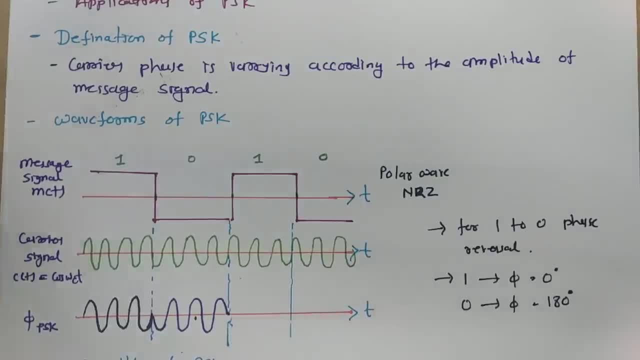 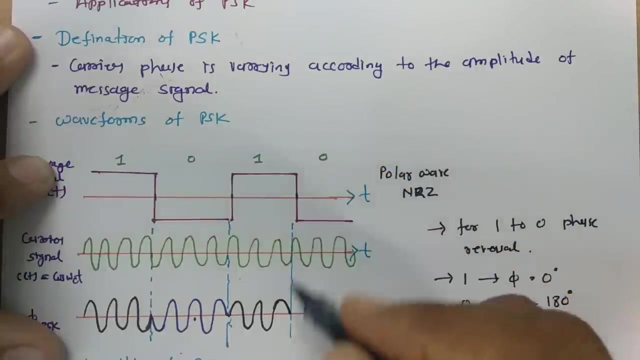 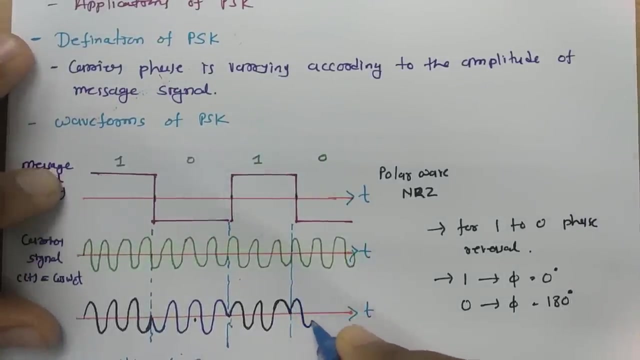 phase reversal. So from here you will be finding there has to have phase reversal. So again you can see over here I have shown phase reversal and for zero now we need to change phase by another 180 degree. So here again there will be phase reversal. 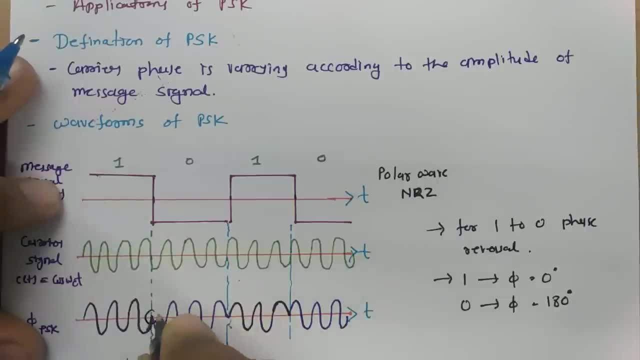 So ultimately, this phase reversal Over here that is happening because of transition of one to zero And here this phase reversal that is happening because of transition of one to zero. Similarly, over here I have shown even phase reversal, So that is happening because of transition from one to zero. 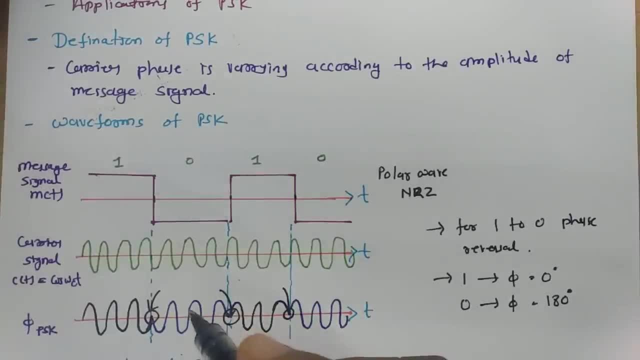 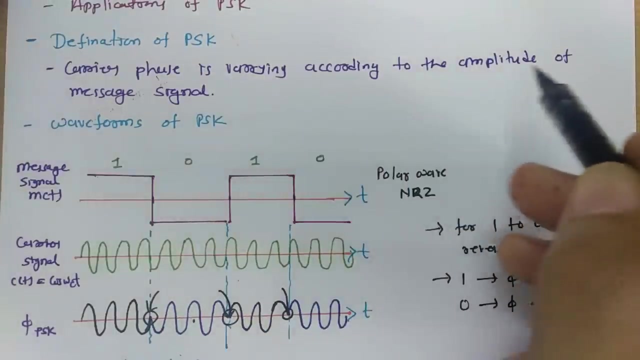 So for binary PSK there will be change in phase by 180 degree, So this is even referred as BPSK, Binary phase reversal, Phase shift King. So ultimately, carrier signal phase is changing with respect to amplitude of message signal. that is what phase shift king. So this is how wave forms are there. 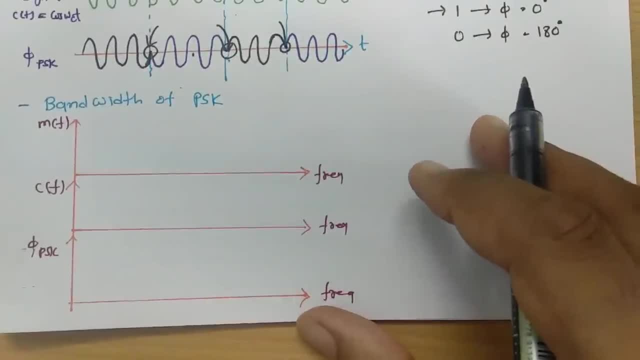 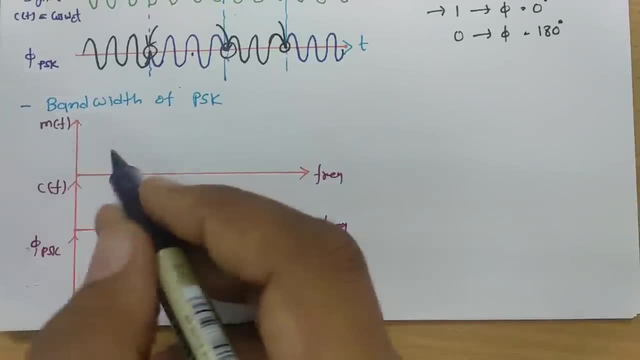 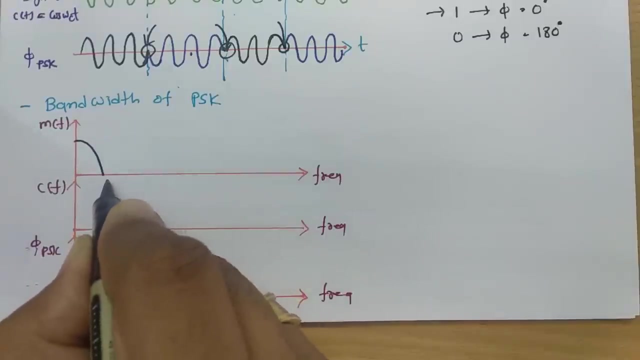 Now let us try to understand bandwidth of phase shift king. So see, we have message signal and in terms of frequency domain I have represented that by MF. If I say its bandwidth, is this much Low frequency signal? How low frequency signal signal is there and its cutoff frequency is FM. We have carrier signal that is high frequency. 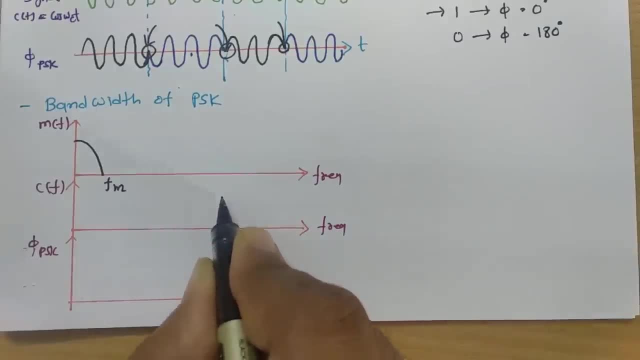 signal and that is sinusoidal signal, So high frequency carrier signal that is having impulse bandwidth, impulse response. The reason is only one: frequency is there and if I say that is FC, then that is how it will be there For phase shifting: by having a center of FC, by having a 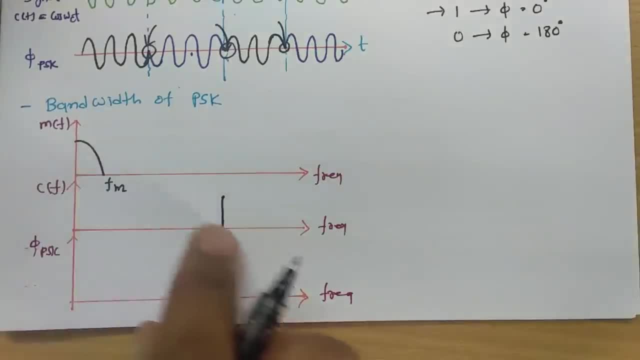 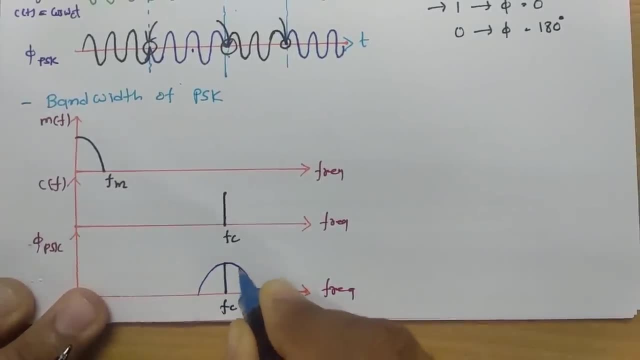 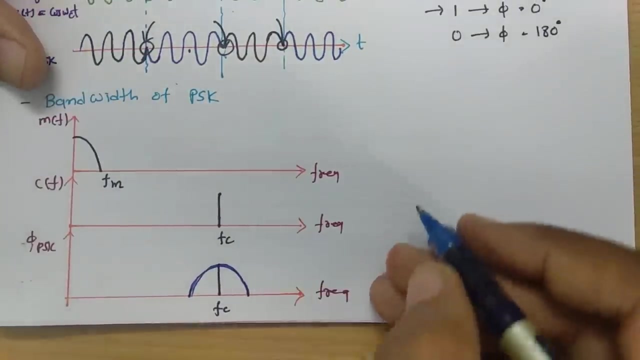 center of FC. we will be molding this message signal onto this So you will be finding. its response will appear like this. Its response will appear like this: and now if I want to calculate bandwidth of this phase shift king, then its bandwidth of PSK that will be proportional to R. 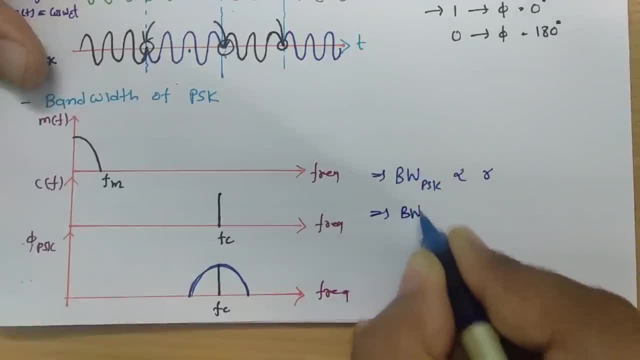 and if you want to calculate what will be that bandwidth, then bandwidth of PSK that is 1. Plus D by R, where D belongs to 0 to 1 for ideal modulation. For ideal modulation D is equals to 0 and for worst case, 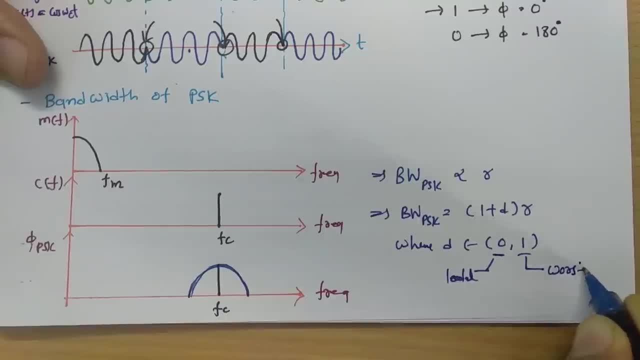 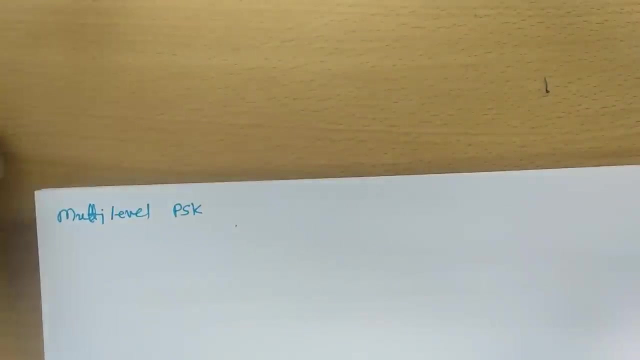 D is equals to 1.. So that is how we calculate bandwidth of phase shift king. That is how we calculate bandwidth of PSK. That is how we calculate bandwidth of PSK. Now let us move on to another part of this PSK session, where now I'll explain what is multi-level. 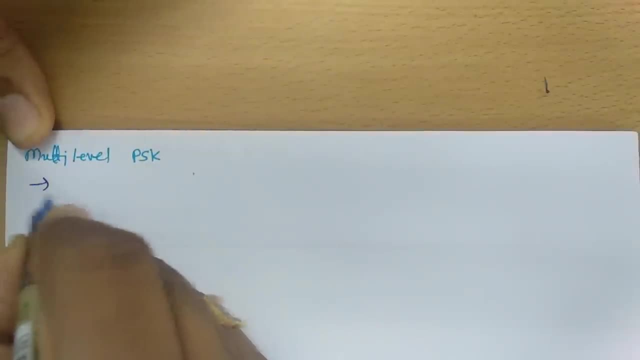 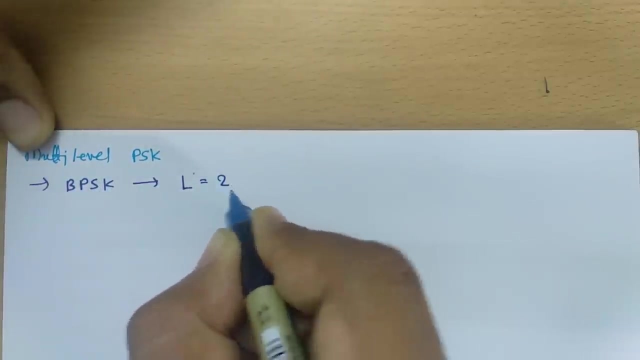 PSK: Now see. I have explained you till now. BPSK: Now see, for BPSK, total levels are: L is equals to 2.. If you compare this with, L is equals to 2, that is, 2 to the power N. then you will be able to see. 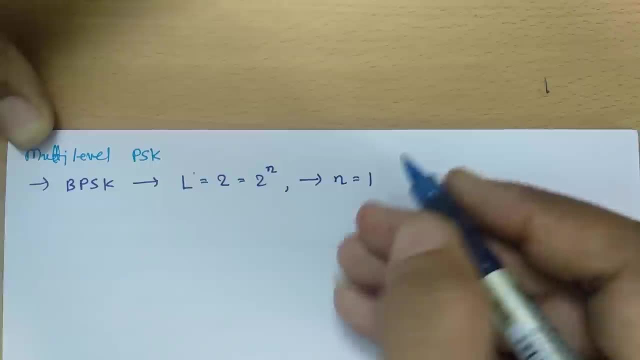 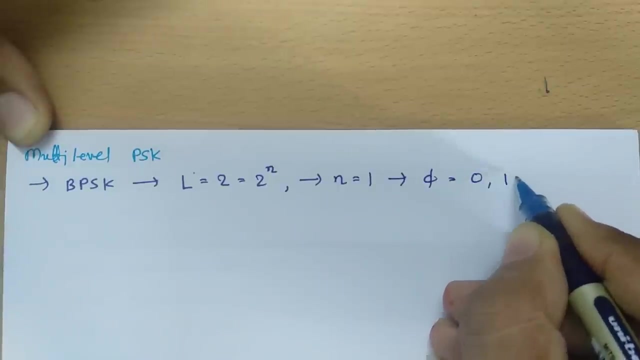 that you will be finding L is equals to 1.. So there are two levels. It means there are two phase. 1 phase is 0 and second phase is 360 by 2. That is 180 degree. So that is how phase will change. now see, if I say I have, L is equals to 4 level. 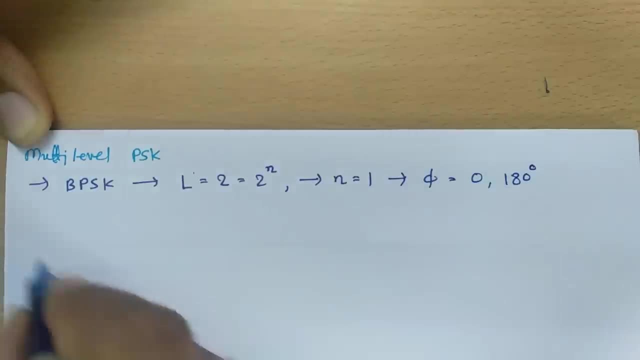 So that is how phase will change. now see if I say I have L is equals to 4 level. So if you compare this with 2 to the power, and then you will be getting N equals to 2.. So for that there are four levels. So 360 by 2 equals to 1.. 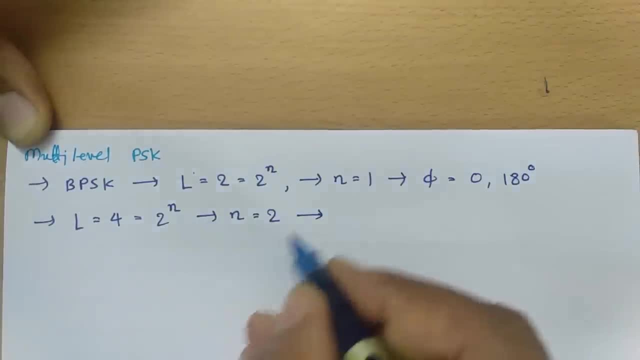 60 by 4 means 90 degree phase for each level will be there. so total phase available will be 0, 90, 180, 270. now see when we talk about L is equals to 8. so in that case if you compare it with 2 to the power n, then you will be getting: n is equals to 3 bit and each level 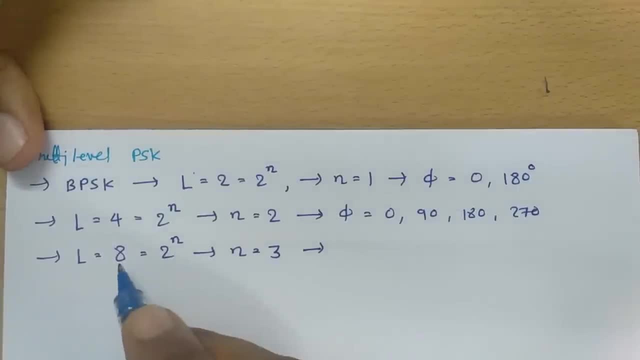 that is having phase which is been changing by 360, by 8 it means it is 45 degree. so total phases for different bits that will be 0, 45, 90, 135, 180, 225, 270, 315. so total 8 different. 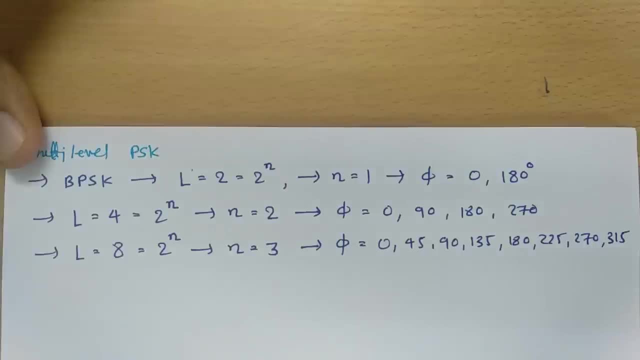 phases are there which will be representing different levels, and that could be representing by 3 bits. so n is number of bits to represent each phase and L is number of levels, which will be showing you how many phases are available to represent particular bits. so that is how. 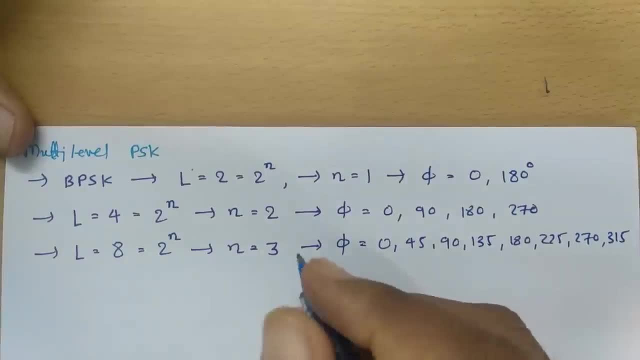 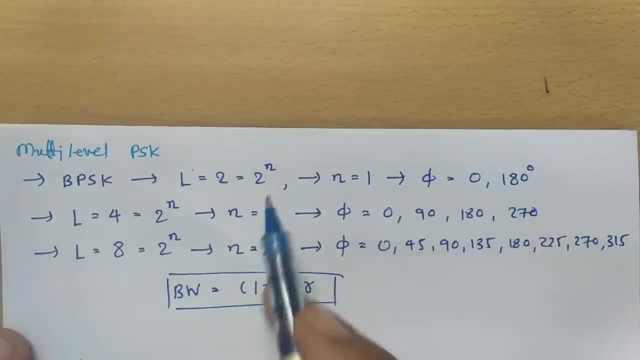 multilevel PSK is there and, as we have seen, its bandwidth, its bandwidth, so that bandwidth, that is 1 plus D into R. that is how we calculate it. So we should remember this for examples. so this is what about multilevel representation of phases and levels with respect to number of bits per level. now let us have a modulation. 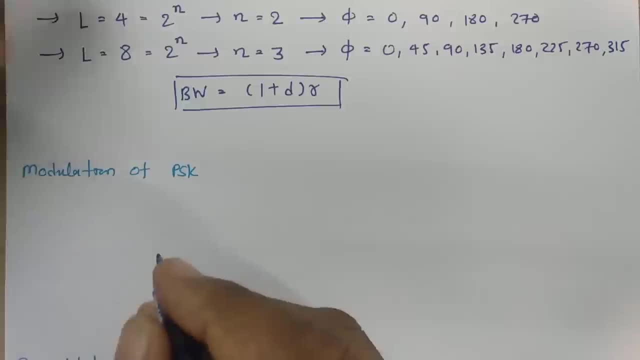 of phase shifting. so when we do modulation, now see, as I have told you, we have a message signal and we have carrier signal, CT. That is cos of omega CT. now see when you multiply these two. when you multiply these two, you will be finding there will be safe phase shifting output and that is plus, or 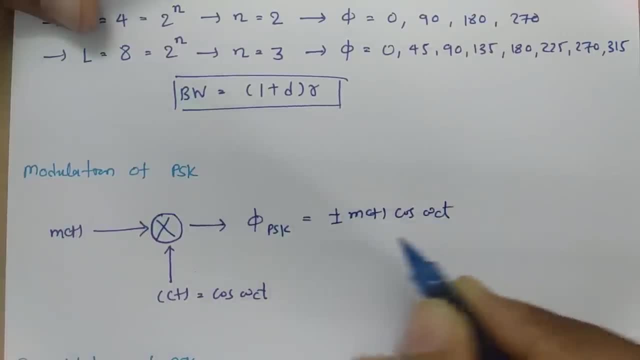 minus mt into cos of omega CT. see, this plus will happen in case of once is there, and this minus will happen in case of zeros. are there, as we have message signal that is digital if you use Polar modulating signal. so polar modulating signal is having plus voltage in case of one. 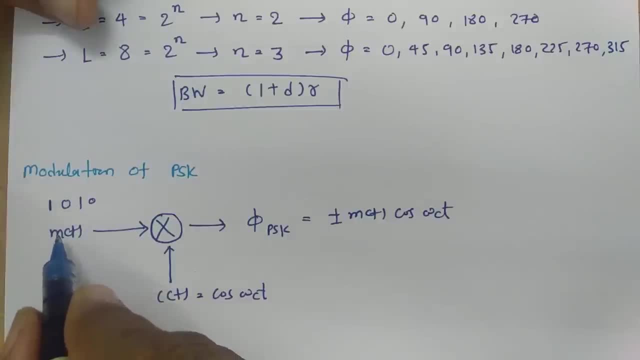 and negative voltage in case of zero. so by multiplying this message signal with carrier signal, we can generate phase shifting output that is plus or minus mt, cos, omega, CT. plus means there is one, minus means there is zero, means there is a phase reversal of 180 degree. 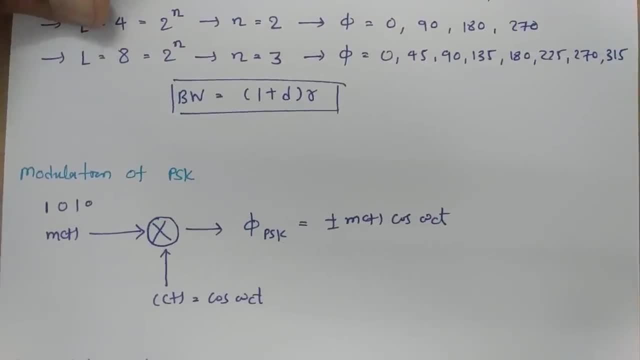 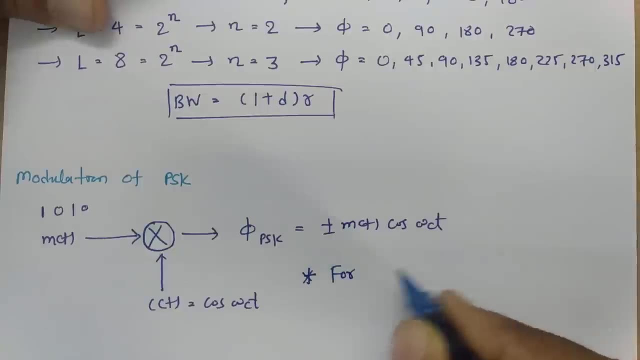 now when we talk about multilevel PSK. so for multilevel PSK, if you want to represent signal for multilevel PSK, then one can represent that by mt into cos of omega CT plus five, where five is phase. now see for four, four level, that five will. 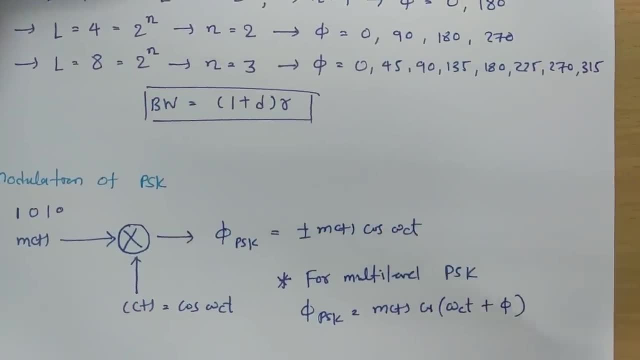 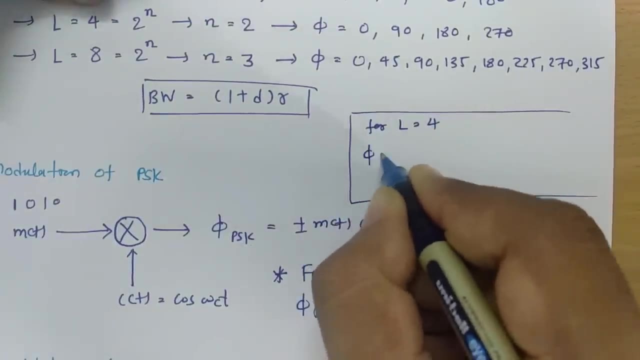 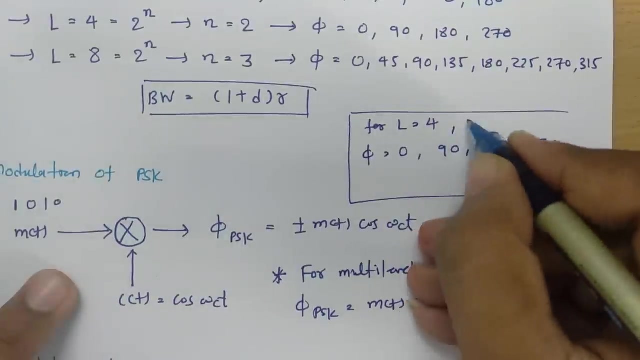 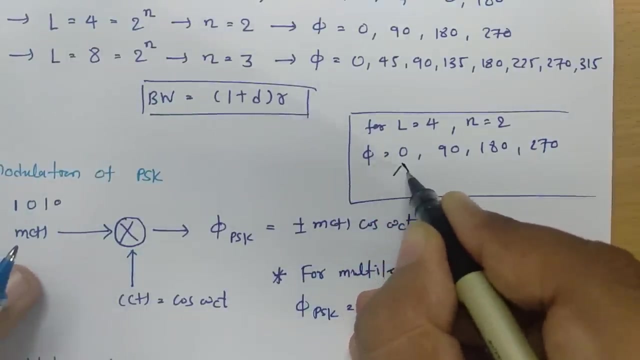 be zero: ninety, one, eighty, Two, seventy. so I'll give you one example over here. so see, four- L is equals to four level- will be having five, that is, zero, ninety, one, eighty and two, seventy, where n is equals to two bits, as we have seen. so to represent zero digitally, it will be zero, zero data to. 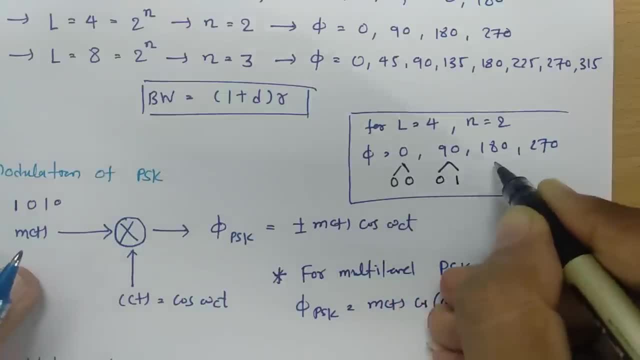 represent ninety digitally, it will be zero one data. To represent 90 digitally, it will be zero one data. To represent 90 digitally, it will be zero one data. To represent phase of one eighty digitally, it will be one zero data. and to have phase. 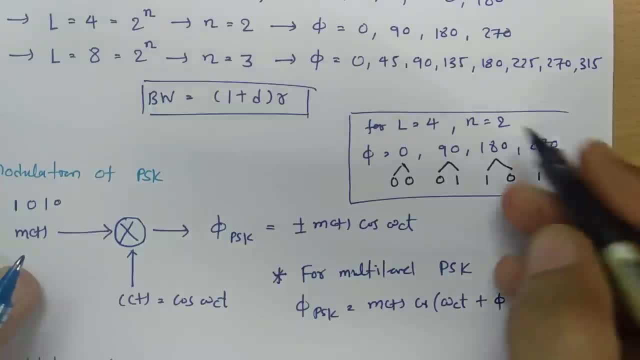 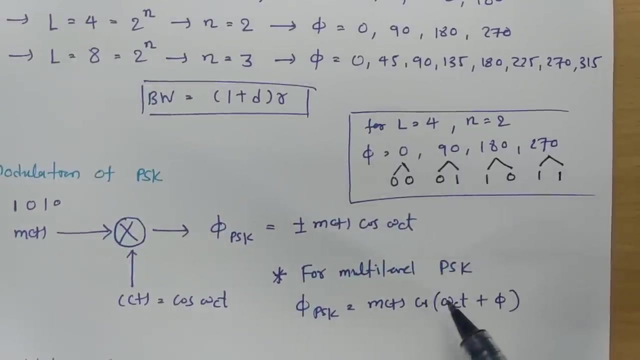 of two, seventy. digitally it will be data of one one, so two bits are represented by each phases and that is what we can place it here for multilevel PSK phase. So we should understand: in phase shifting we change phase of carrier signal with respect. 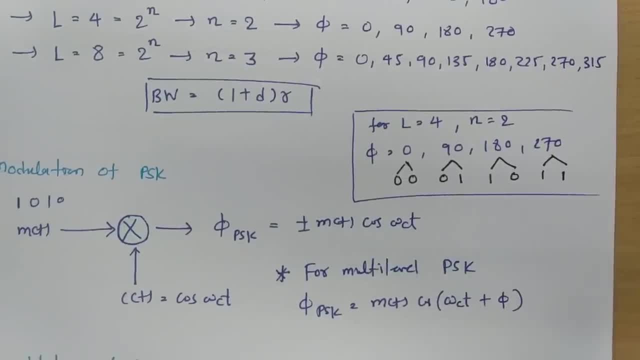 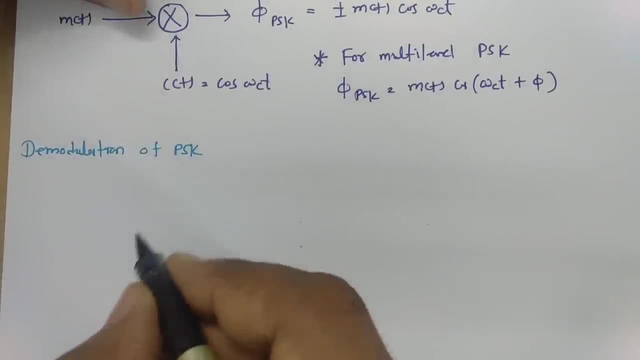 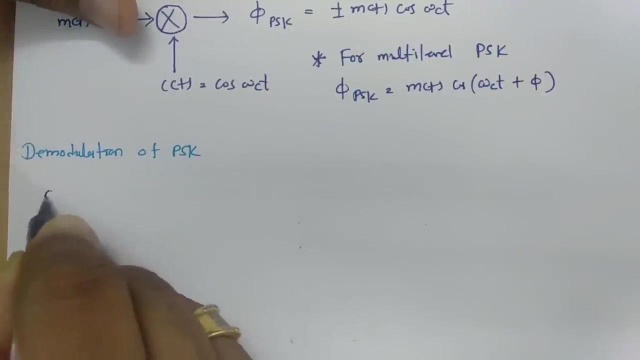 to amplitude of modulating signal. Now let us have demodulation of phase shifting. So demodulation of phase shifting, so that is what? as similar as we see it in ASK and FSK. so in that we will be receiving PSK signal. 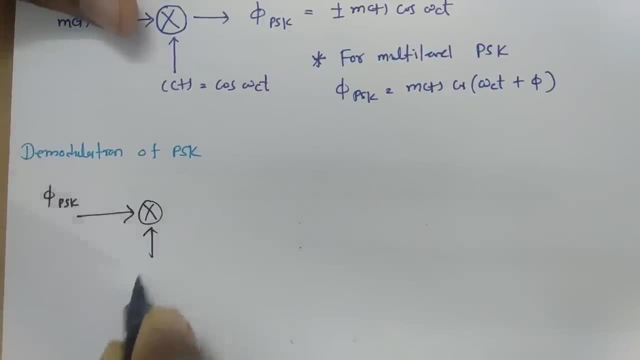 Now all we will be doing is we will be multiplying it with carrier signal. this is what coherent demodulation. this is what coherent demodulation, where we use carrier signal and after multiplying, after multiplying, if I say I have a signal yt, then this yt signal, this yt signal, so that has to be phi of psk. 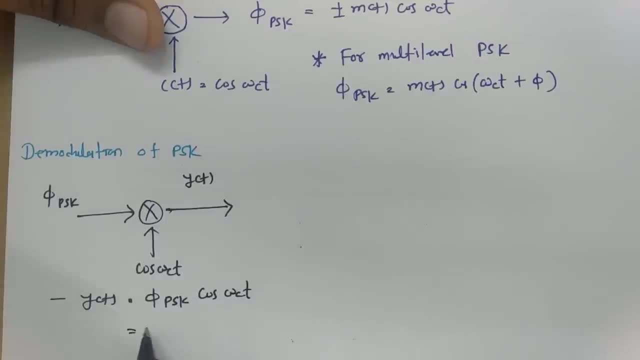 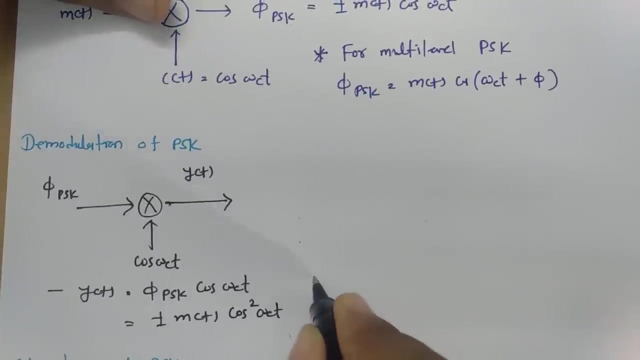 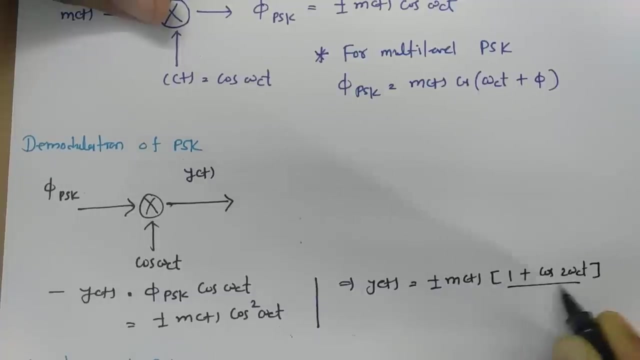 into cos of omega ct. Now, what is phi of psk? Phi of psk, that is plus or minus mt, cos of omega ct, into cos of omega ct, that will be omega ct square. and if you further simplify this, then this yt, that is plus or minus mt, into 1 plus cos 2 omega ct, and this divide by 2.. 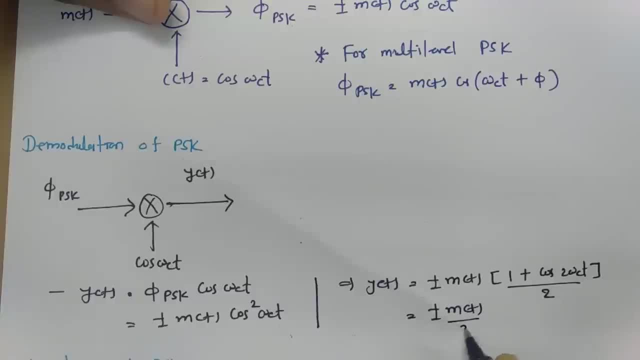 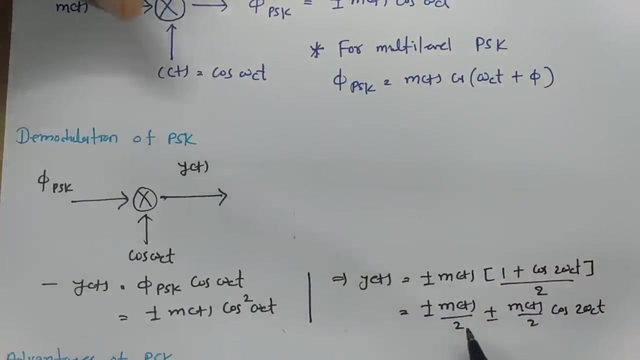 So you will be having plus or minus mt by 2, plus or minus mt by 2 into cos of 2 omega ct. So this is what the yt which we will be having Now here one can clearly see. this is my information, This is my data and this is high frequency component. So to remove this. 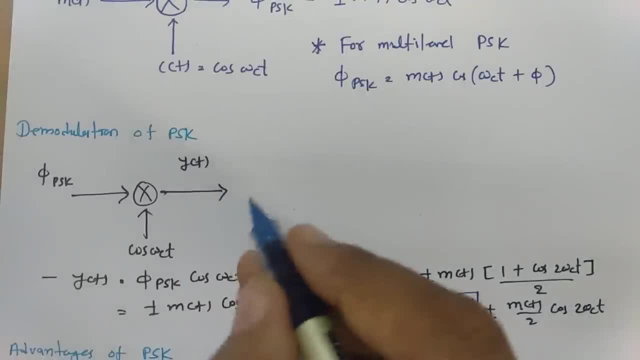 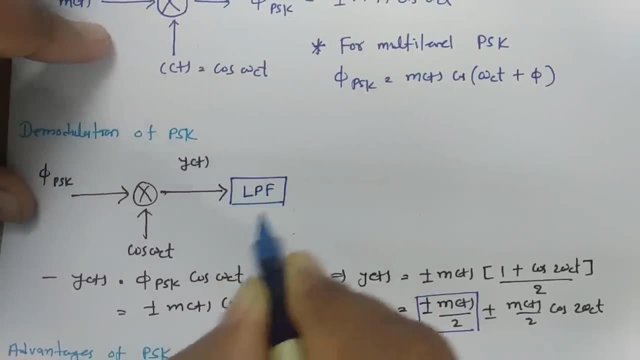 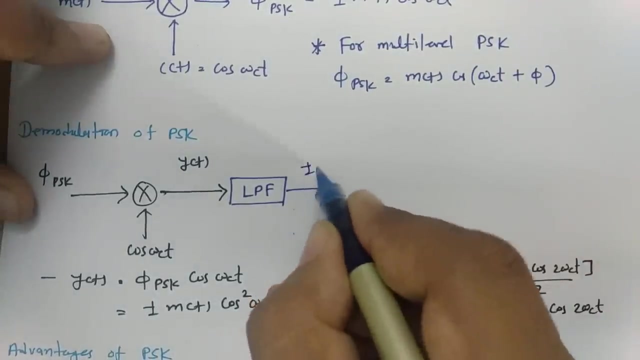 high frequency component. we can pass this yt through low pass filter. So here, if I pass this through low pass filter, Here, if I pass this through low pass filter, my output that will be plus or minus mt. So here now I will be having output. 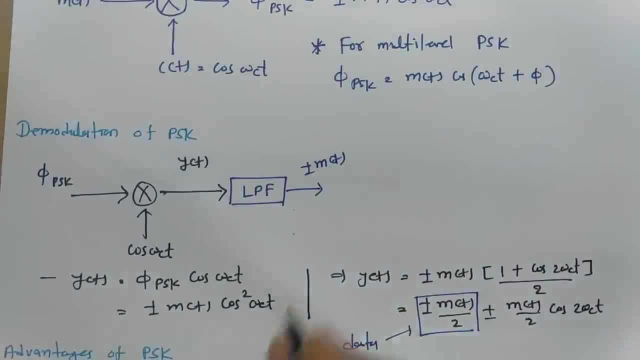 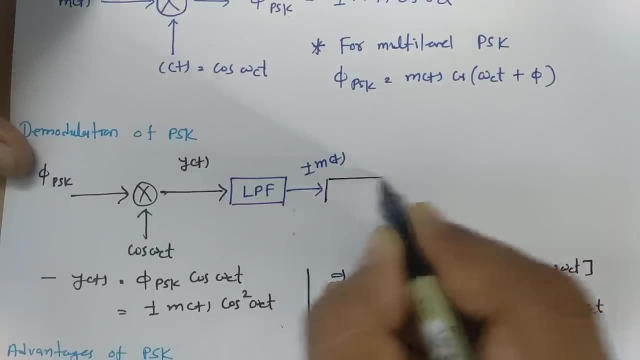 that is plus or minus mt. Now see, we have output that is plus mt or minus mt. So to get exact data mt, we need to pass this signal through decision making device or comparator, So we will be having exact output. So if you pass this signal through comparator, you will be extracting original. 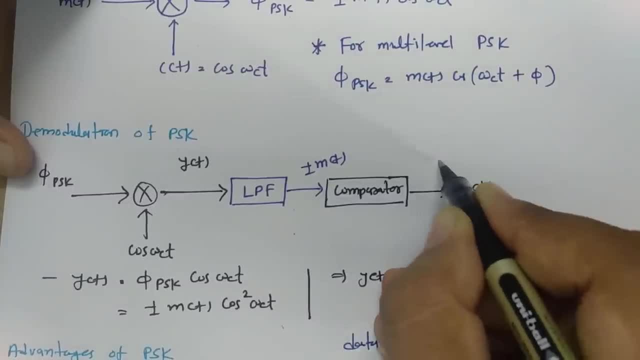 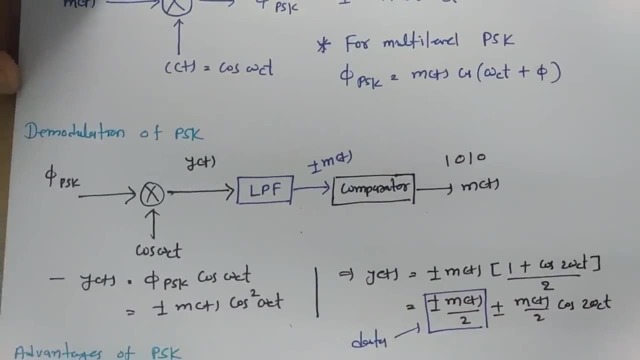 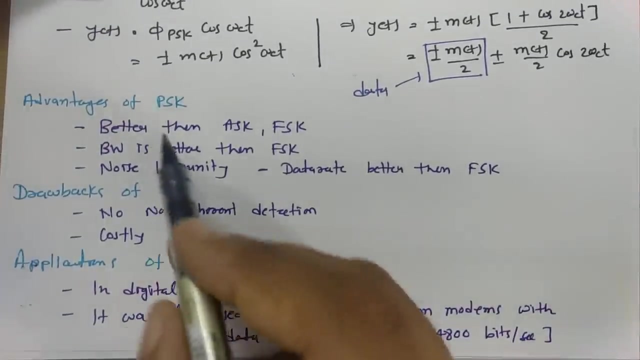 information and that will be mt. Now mt will be there in digital data: 1 or 0. So this is how we do demodulation of phase shifting. I hope that you have understood this. Now let us sum up this session with advantages, drawbacks and applications. So see, advantages, are it? 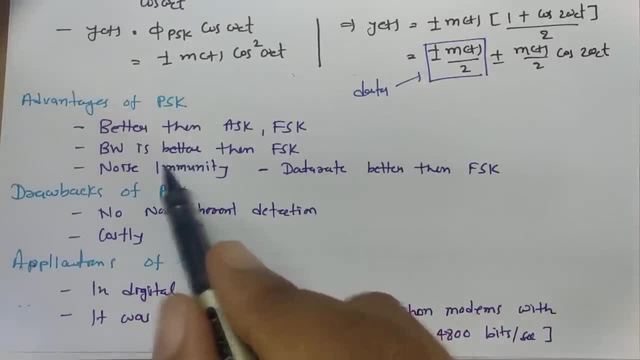 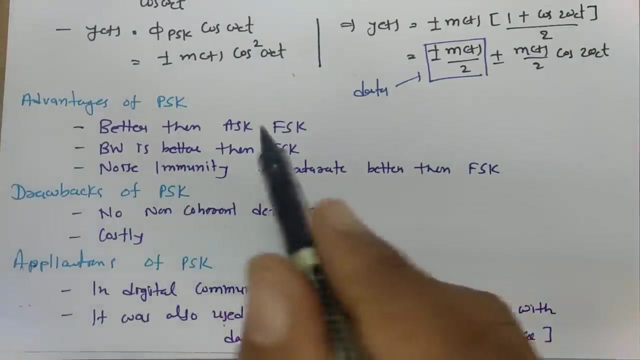 is better than ASK and FSK. Bandwidth is far better than FSK, Noise immunity is good and data rate is better than FSK. When we talk about drawbacks of phase shifting, we have added more then lane passatley 3.3 Phot animation. it is now less than that and ANOVA increased.